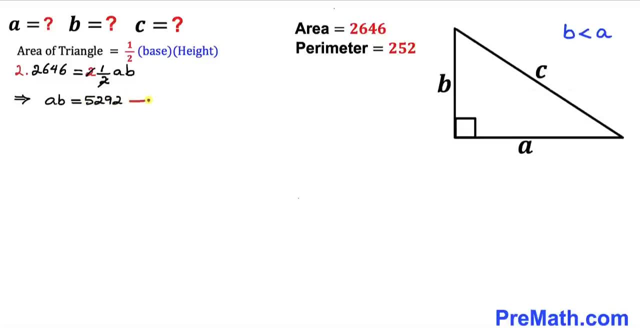 Let's go ahead and call this our equation number one and here's our next step let's recall the perimeter, the perimeter is the sum of all these boundary lengths. So that means perimeter is going to be a plus b plus c and in our case the perimeter has been given to us as 252. So let's go ahead and fill in the blanks in this equation. So therefore our a plus b plus c value turns out to be 252. Let me call this as equation number 2. And here's our next step. Let's recall the Pythagorean theorem. Since we are dealing with this right triangle, Pythagorean theorem is a square plus b square equal to c square. 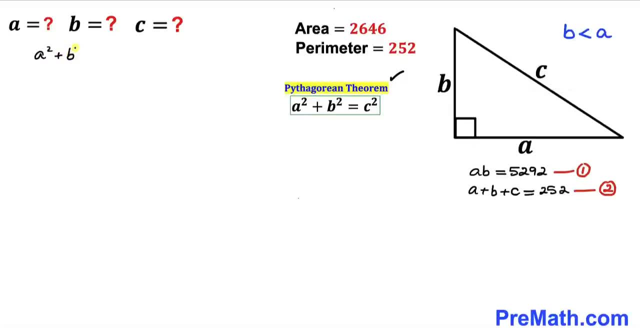 Let me go ahead and write down a square plus b square equal to c square. Let me go ahead and call this our equation number 3. 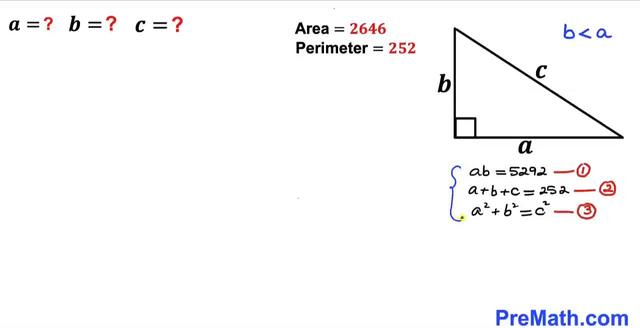 And now as you can see we got this system of three equations. And now we are going to solve this system to calculate the value of a, b and c. And now let's focus on this equation 2. And here I have copied it down. Let's go ahead and write down a plus b square equal to c square. Let's go ahead and move this c on the right hand side. 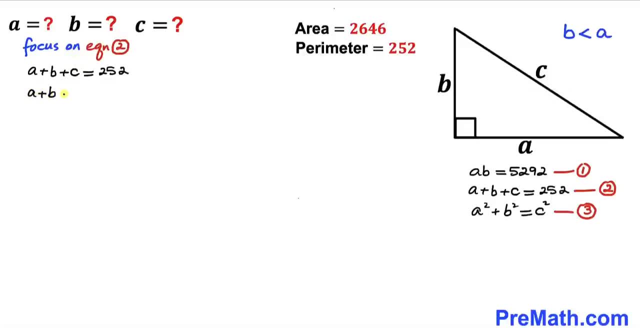 So therefore we are going to have a plus b equals to 252 minus c. 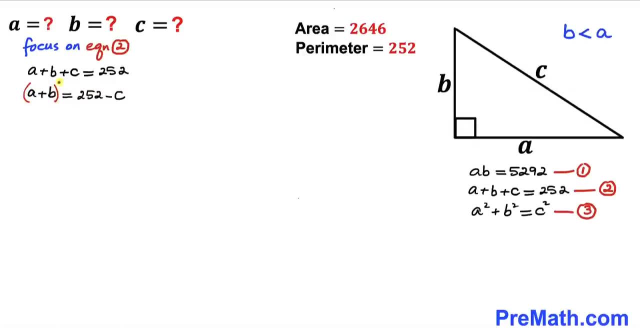 Now let's go ahead and take a square on both sides. We are going to manipulate this one now. 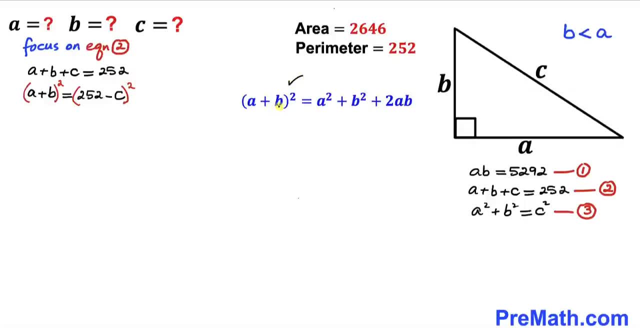 And now let's recall this famous identity a plus b whole square. I'm going to apply it on the left hand side. So I can write a square. 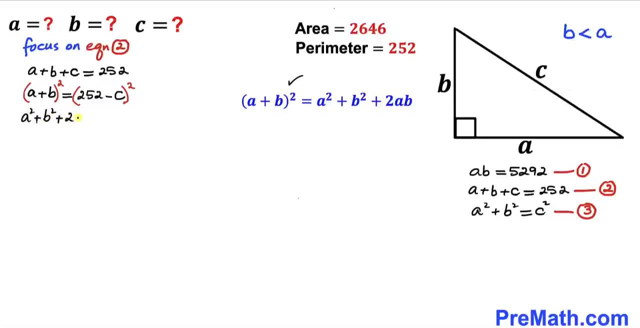 Plus b square plus 2 times a b equals to. 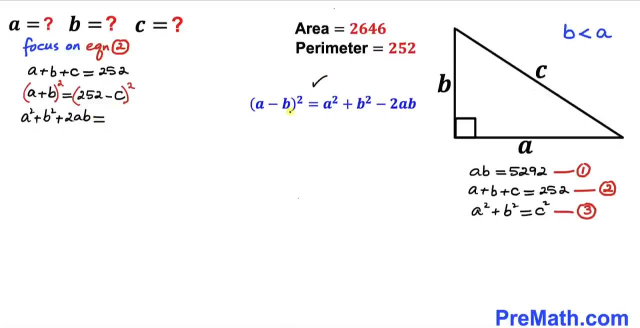 And now let's recall this another identity a minus b whole square. We are going to apply it on the right hand side. So the right hand side is going to become the square of 252 is 63504 plus c square minus 504c. 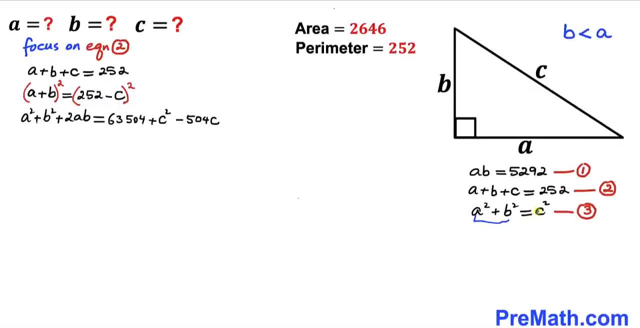 And now we can see a square plus b square equal to c square. So therefore I'm going to replace this a square plus b square by c square. 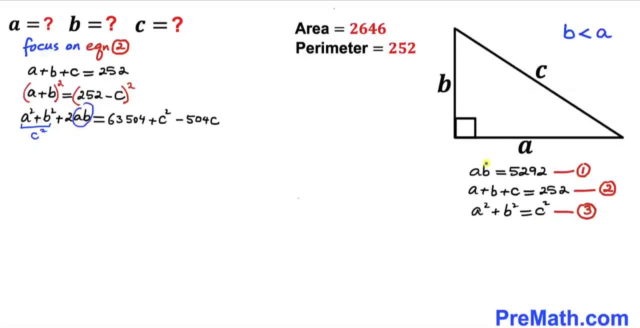 And likewise this a times b I am going to replace this a times b equals to 5292. So this is going to become 5292. As you can see in this next equation I have replaced this a square b square. So this is going to become 5292. So this is going to become 5292. And likewise I replace this a b by this 5292. 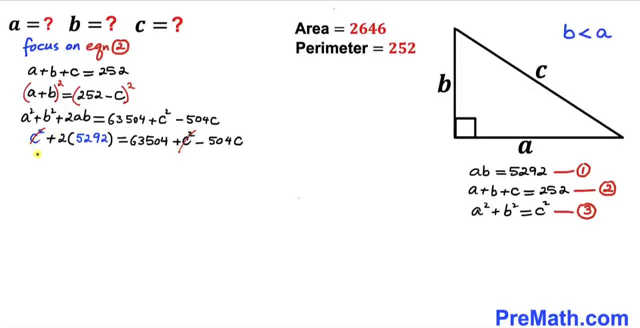 And now we can see this c square and c square on both sides they cancel each other out. 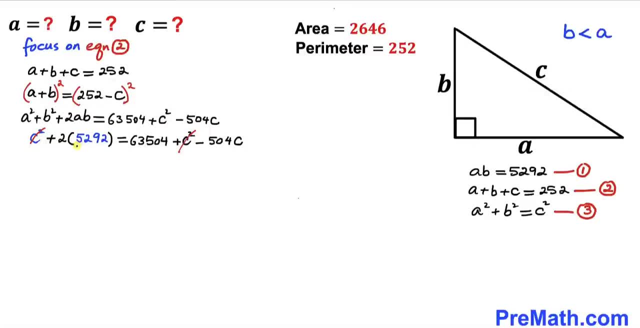 And now let's go ahead and simplify furthermore. So 2 times 5292 is going to give us 10584 equal to 63504. 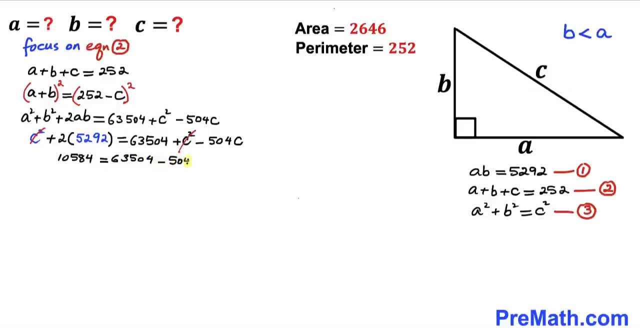 And now let's go ahead and move this negative 504c on the left hand side. And at the same time I'm going to move this 10584 on the right hand side. 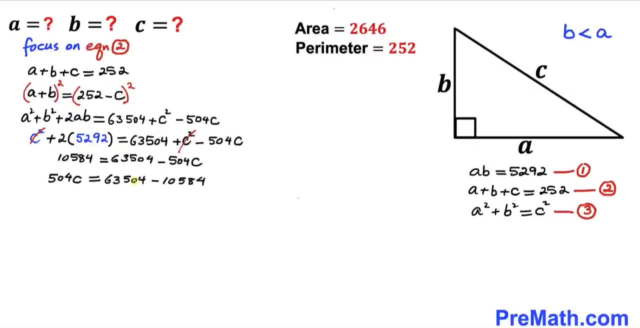 As you can see in this next equation. Now let's simplify furthermore. 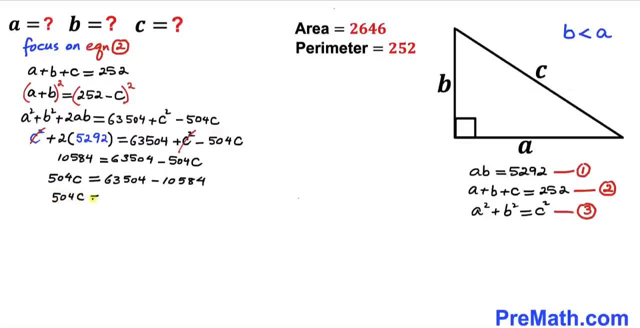 So 504c turns out to be 52920. 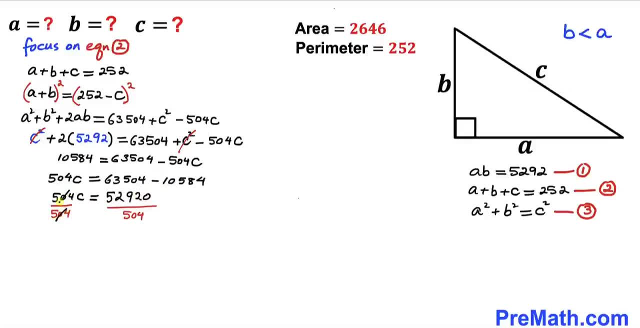 now let's divide both side by 504 on this side this is gone so therefore our C value turns out to be 105 so thus our C value turns out to be 105 and now 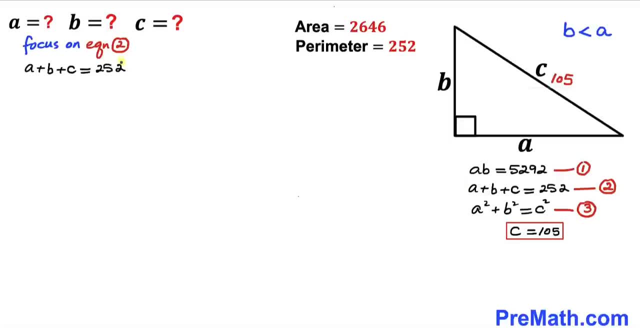 let's focus on this equation 2 once again and here's our equation 2 and now we know that C value is 105 that we just figured out I'm going to replace this one by C over here 105 so therefore we're going to have A plus B plus C I'm going to replace it by 105 equals to 252 and now let's go ahead and 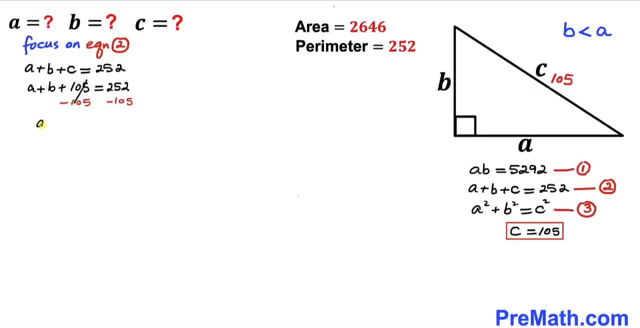 subtract 105 from both sides this is gone so our A plus B value turns out to be 147 and here's our next step let's focus on this equation 1 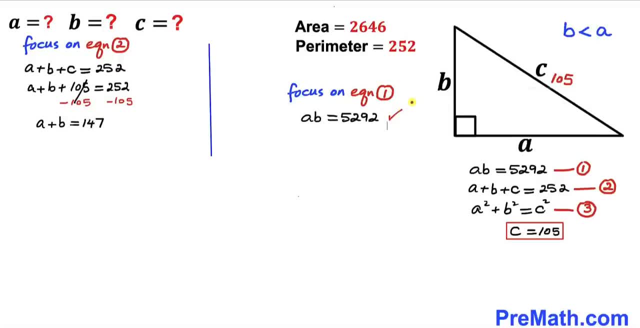 and here I have copied down this equation 1 now let's go ahead and divide both sides by A I'm gonna divide A on this side and A on this side and we can 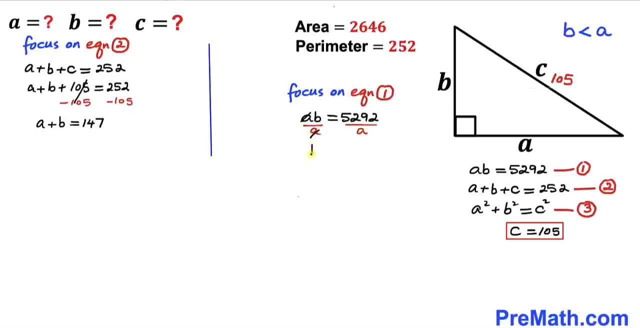 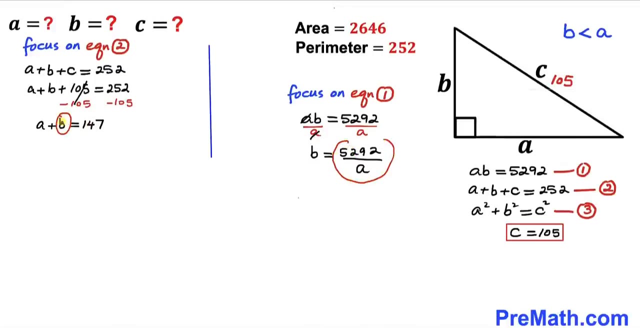 see that this共 diferença A and A is gone so our B value turns out to be 52 92 divided by A and now I am going to substitute this B value over here in this equation over here as you can in this next step I have replaced this b by this value as you can see over here and now we are 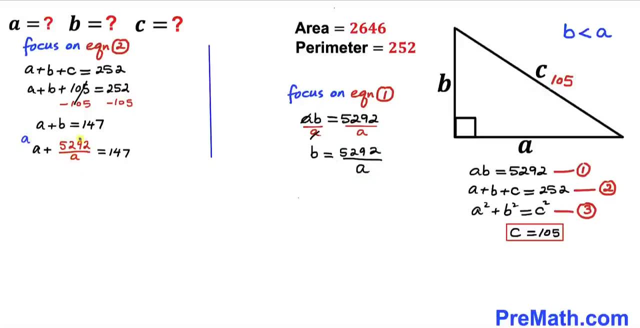 going to remove this fraction so I'm going to multiply all the way across the board by a so here a times a is going to give us a square here a and a is gone so we got plus 52 92 equals to 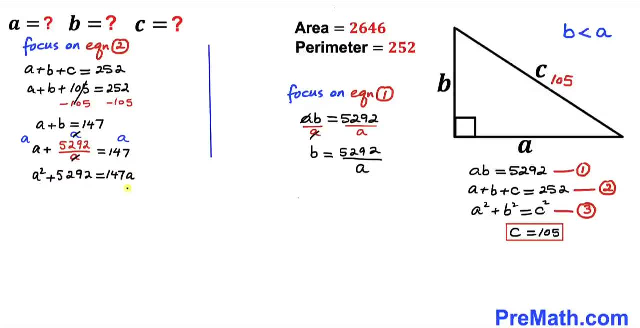 147 a and now let's go ahead and move this 147 a on the left hand side as you can see in this next step I have moved this 147 a on the other side and it became negative 147 a and now we can 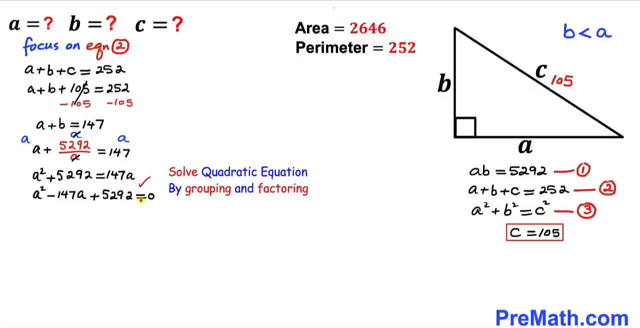 see that this is our quadratic equation and we are going to solve it by grouping and factoring now let's focus on this 52 92 and here we are going to multiply all the way across the board 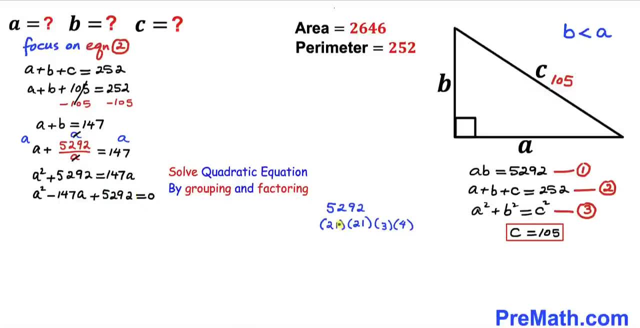 here I have copied it down and if we pay a little attention we can see that this could be broken down to 21 times 21 times 3 times 4 so let me go ahead and rearrange this thing 21 times 3 is going 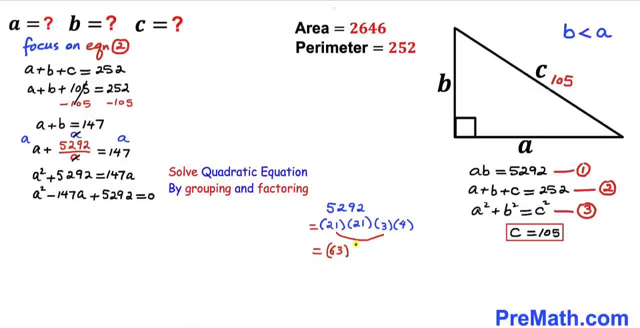 to give us 63 and likewise 21 times 4 is going to give us 84 so therefore let's focus on this middle number negative 147 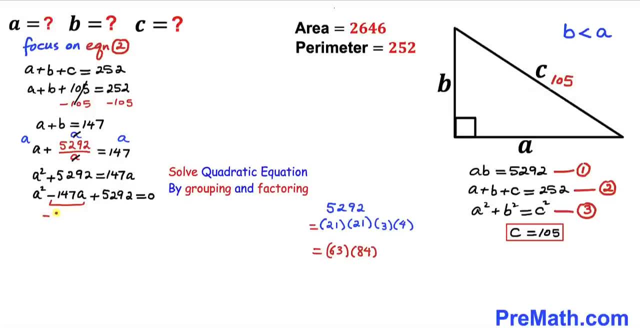 a I can tweak this thing I can write this thing as negative 63 a minus 84 a it doesn't make any difference whatsoever as you can see in this next step I have replaced this negative 147 a by this and now we can see between first two terms a is in common and between these last two terms negative 84 is in common so therefore I can 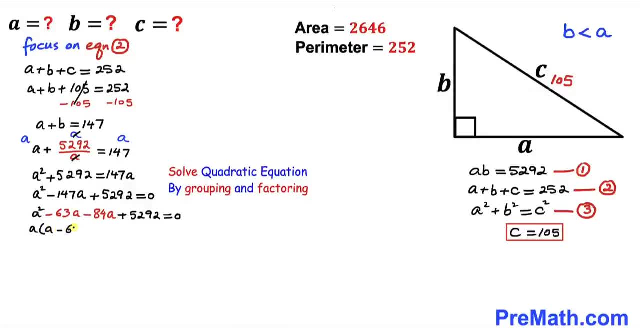 write a times a minus 63 minus 84 in common so we got a minus 63 equal to 0 and now we can see a minus 63 and a minus 63 is in common so therefore we can write a minus 63 times a minus 84 equal to 0. Let's go ahead and break this down. 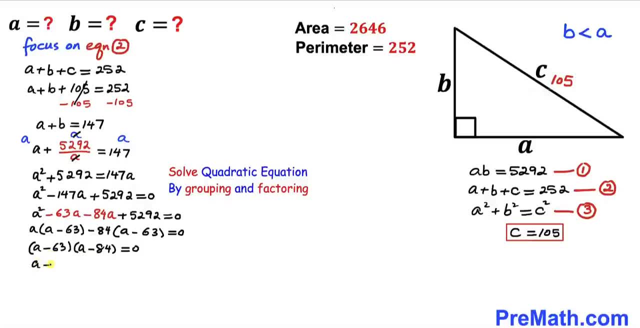 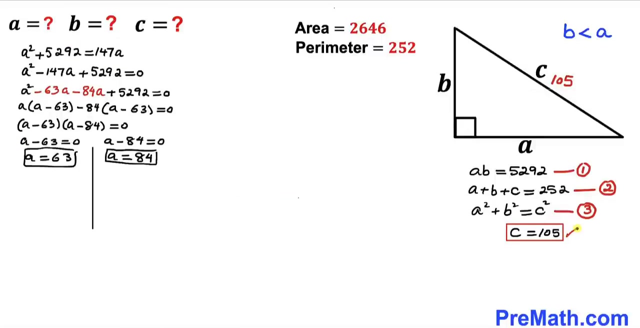 it down so i can set a minus 63 equal to 0 and the other one is going to be a minus 84 equal to 0 and here in the first equation a is going to give us a positive 63 value and for the second equation a is going to be positive 84 value and now we see that we got our c value is 105 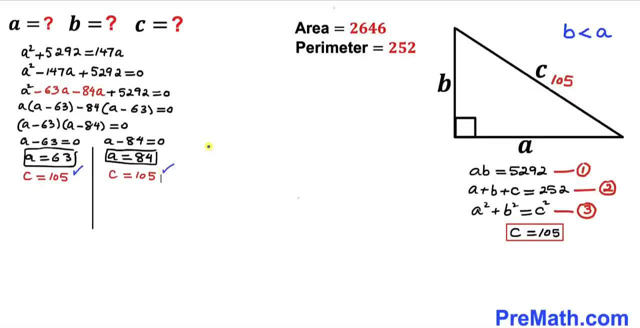 and here i have copied down c value on both sides now we are going to calculate the b value in both scenarios and now let's focus on this equation too 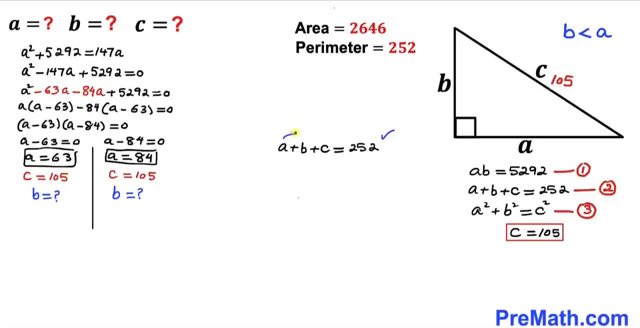 and here i have copied down let's go ahead and move this a and c on the right hand side to isolate b as you can see in this next step now let's focus on this first scenario our a 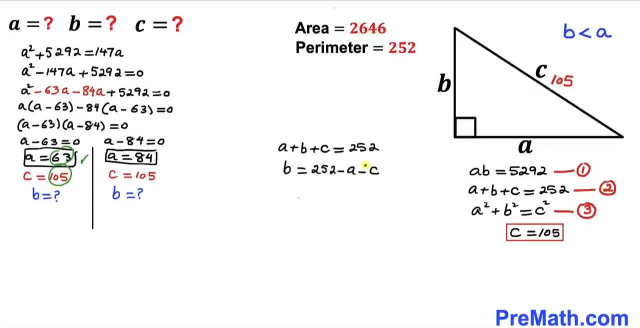 is 63 and c is 105 i'm going to replace these values over here for 63 and 105 as you can see in this next step so if we simplify the right hand side b value simply turns out to be 84. 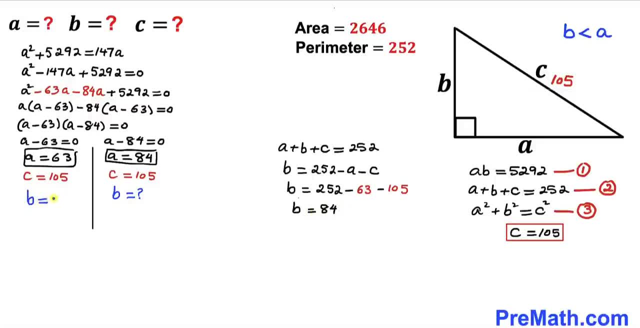 so therefore for this scenario b value turns out to be 84. now let's focus on this second scenario our a value is 84 and c value is 105 i'm going to replace this a by 84 and c by 105 as you can see in this next step let's go ahead and simplify so b value turns out to be 63 therefore for this 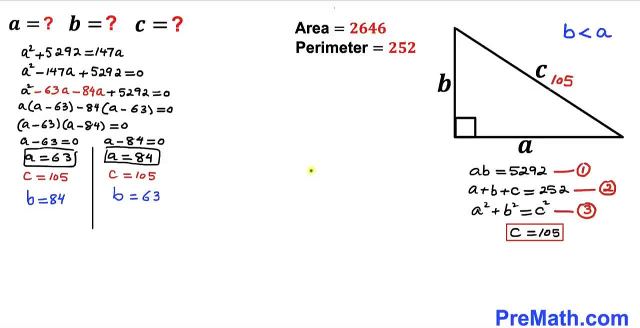 second scenario b value turns out to be 63 and now let's recall our condition b must be less than a and in this first scenario b is not less than a so we are going to reject this scenario and we are going to accept this second scenario so therefore our a value turns out to be 84 and b value is 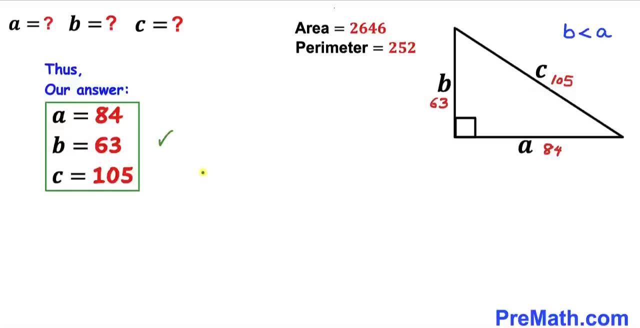 solution thanks for watching and please don't forget to subscribe to my channel for more exciting videos bye 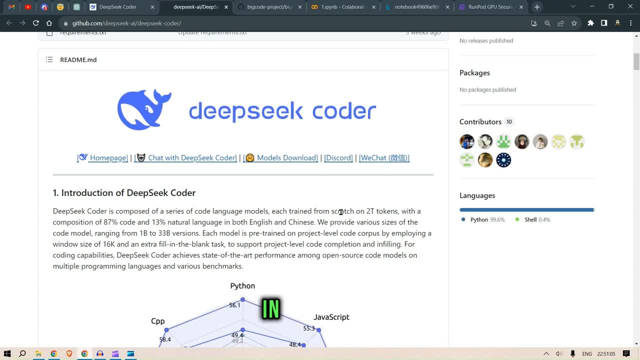 hi guys sorry for the scary thumbnail in this video we are going to go deep dive into deep seek coder llm now i would not like to claim that this is the best 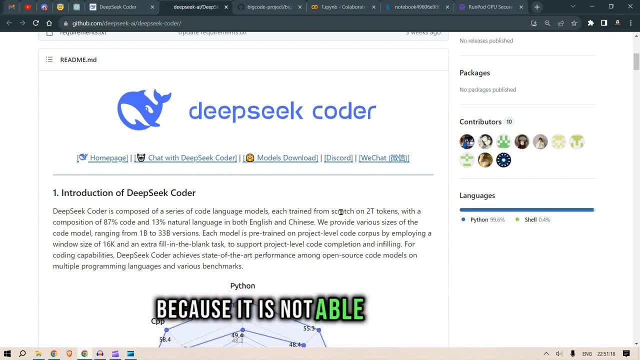 coder model out there because it is not able to beat gpt4 but it is the best in the open source world it is also able to compete with gpt 3.5 turbo 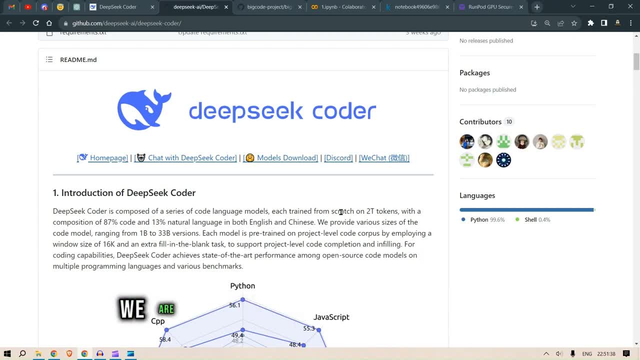 let's look at the model but in this video we are going to approach the problem in a 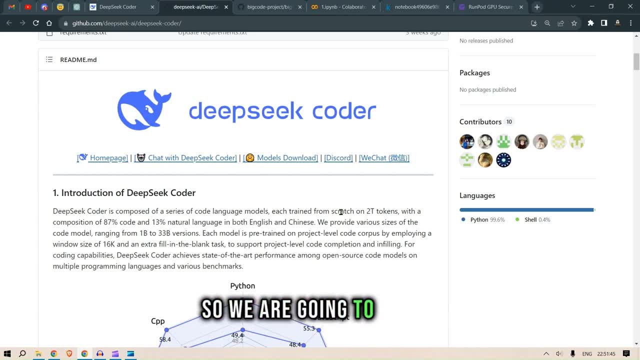 slightly different approach so we are going to try to keep in our minds the ways how the researcher has done the modeling of this model how the data has been trained and what aspects the authors have put to make this model and we are also going to